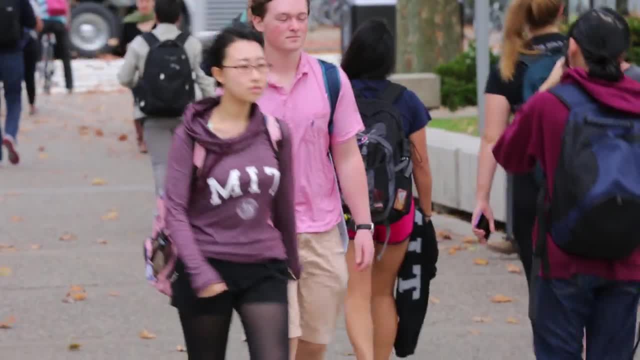 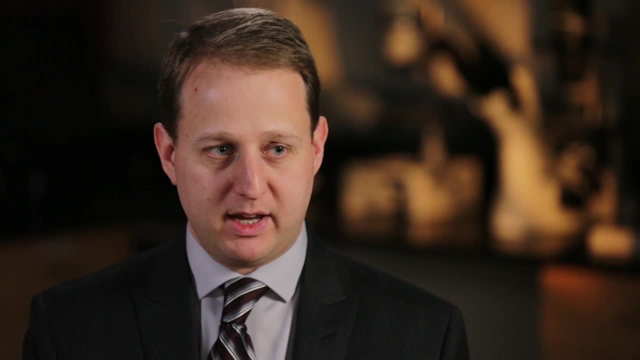 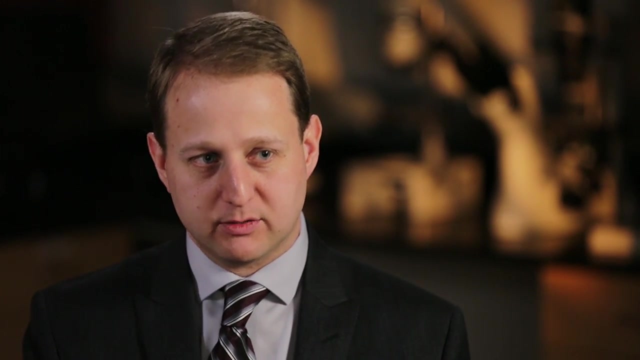 efficient than one-to-many delivery of content, right? So the lecture model where one person delivers to hundreds of people that kind of content can increasingly be made compartmentalized in online modules where students can not only sit one time through a lecture delivered. 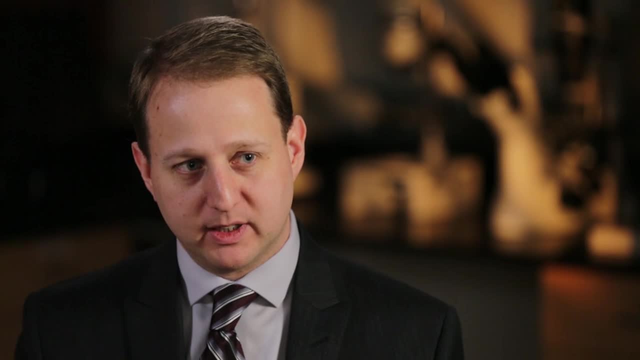 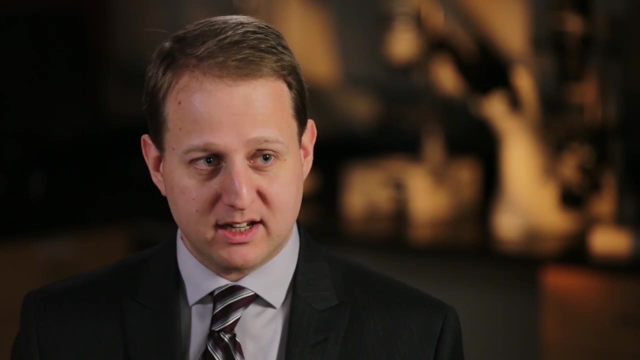 at them, but they can watch it over and over again. It can be hyperlinked to appropriate text materials and reference materials, and it can be available 24 hours a day, seven days a week. So, for instance, I teach a course on the mechanical behavior of materials and I've been teaching 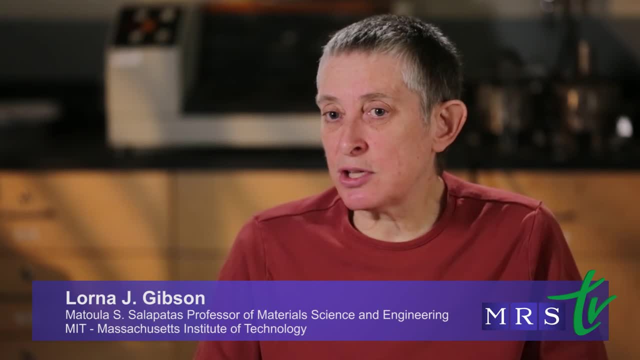 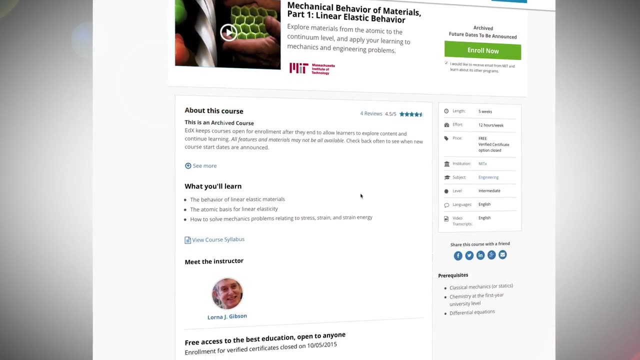 that for many years here at MIT. I've also developed it as an online course through MITx and edX. So to do that, we videotaped the lectures. I developed screencasts of examples, a little like the Khan Academy, I worked out examples on a tablet so students could see. 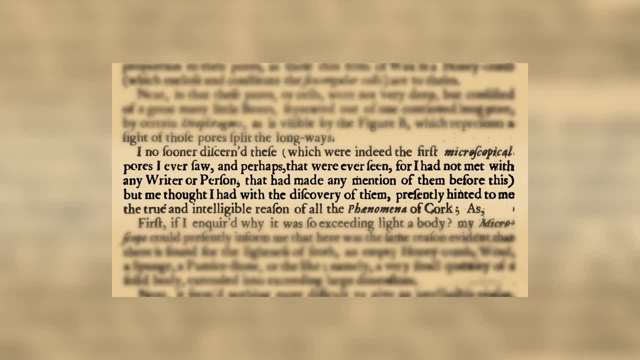 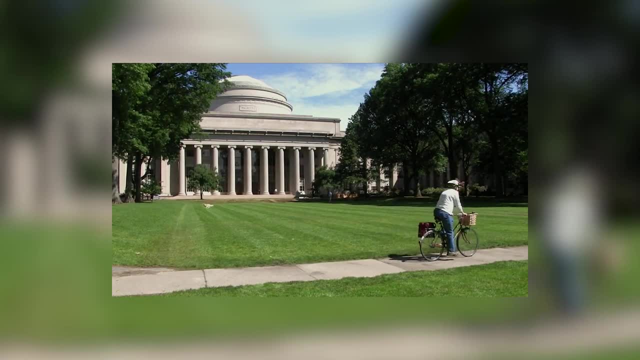 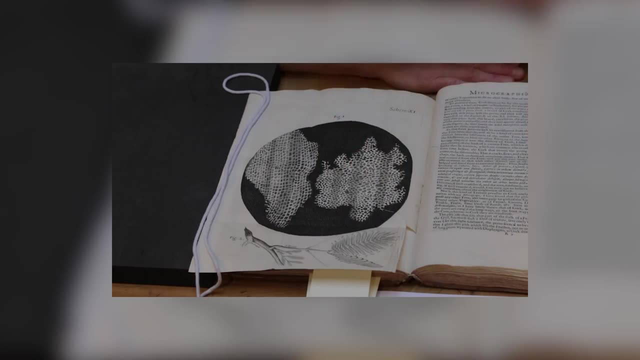 that And all of these things that I developed for the online outside education for people outside of MIT is also available for the MIT students. The online students outside of MIT have been very enthusiastic and they've been very appreciative of what MIT has done here. I think people are a little stunned and amazed that MIT is. 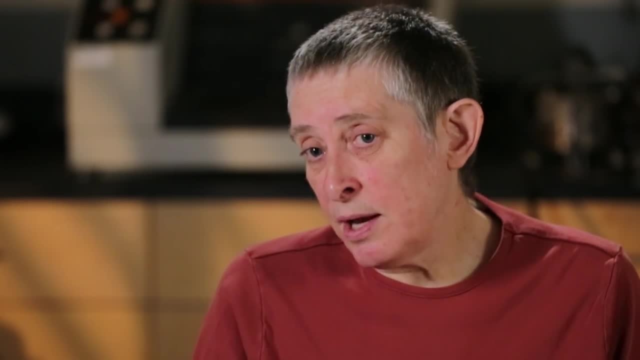 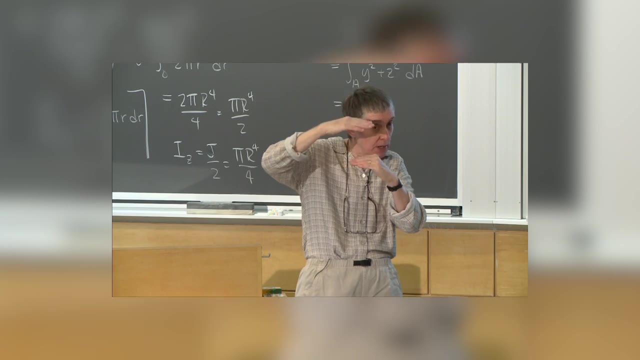 making all this material available and that the quality of what's offered is so good. I've been impressed with how many different countries the students have been from who are taking the online courses. My mechanical behavior of materials class, which was taught last fall, had students from 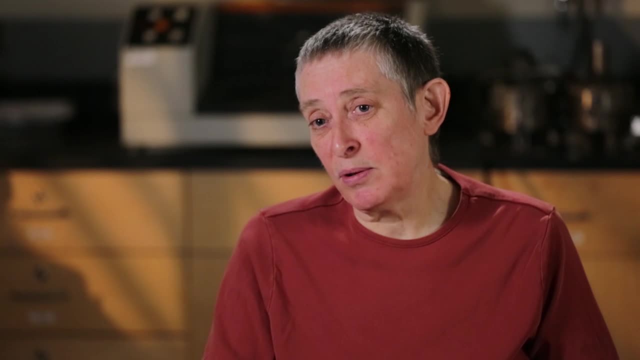 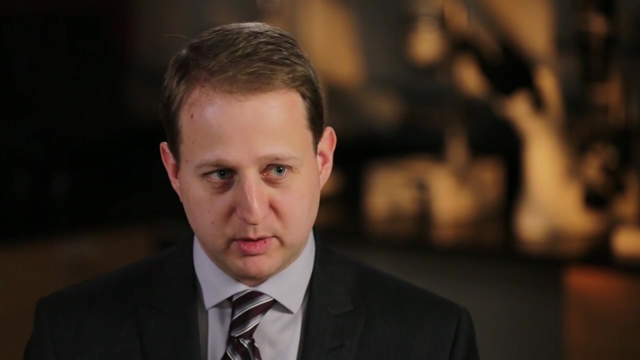 over 140 countries taking it, and I thought that was really remarkable. One of the things that we love in material science and engineering is that when you've gone to the trouble of designing and constructing a new material, new materials can be used in lots of different ways, And so it's pretty common that we might be designing a material. 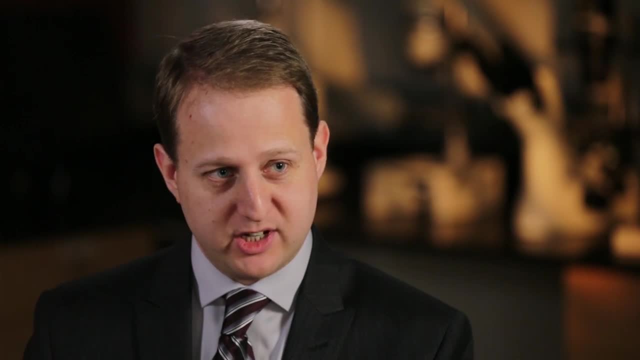 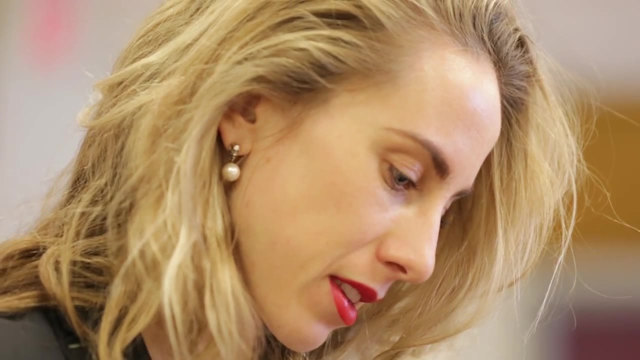 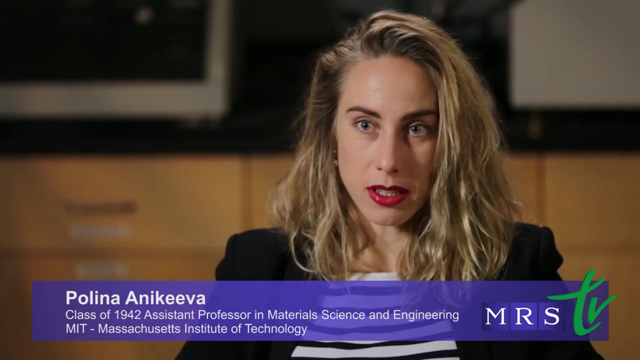 for one application and we find that it's a platform technology and it can be applied broadly across a whole range of industries. Our lab is interested in manipulating and recording neural activity in both the brain and the spinal cord, and also peripheral nerves, And in order to do something like that, you 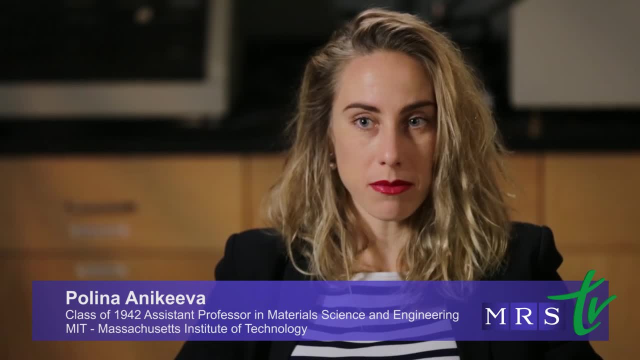 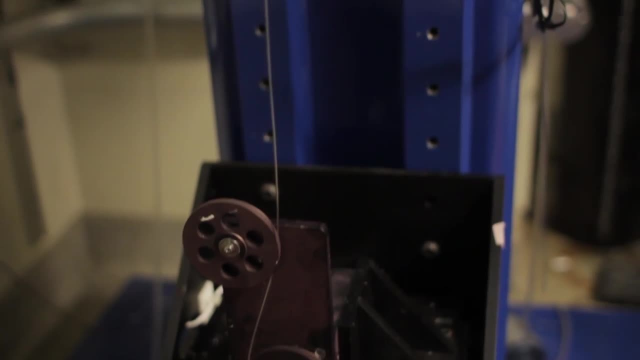 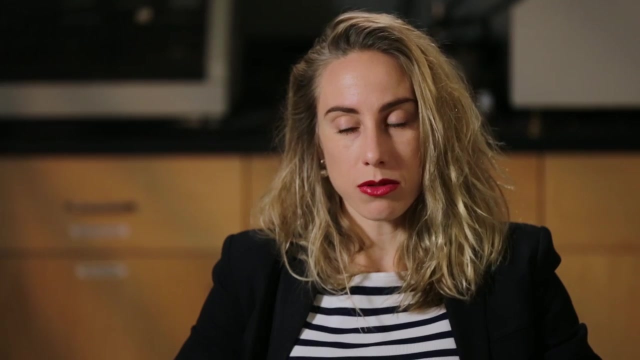 need a device that is flexible so it can address the mechanics and materials properties of the neural tissue. We decided to leverage multi-material fiber technology, which was largely pioneered by Professor Joel Fink, also in our department, except that we decided that we needed to use really soft materials. 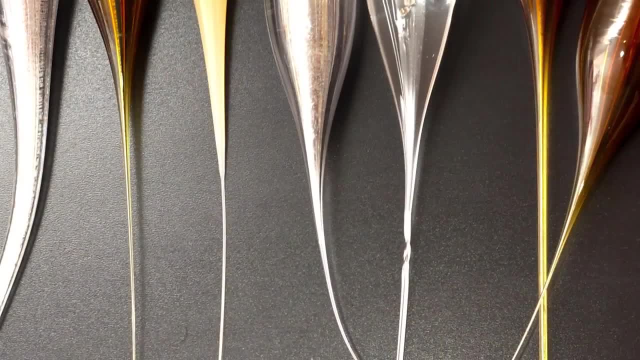 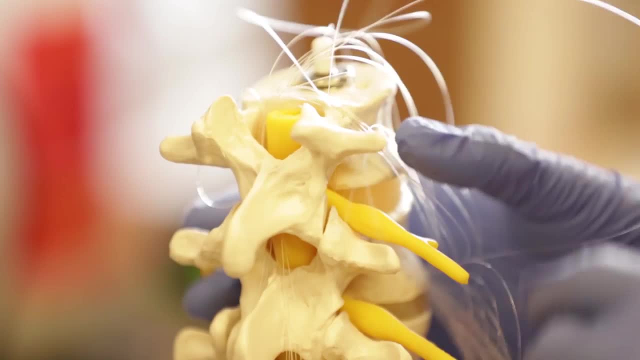 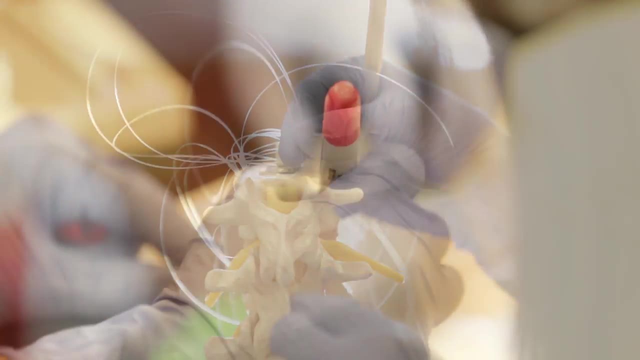 Most of them are polymers and polymer composites, And then we can introduce all of these materials into a structure which is a template of the device and we can now implant it into the brain or the spinal cord or peripheral nerves and interact with that complex system minimally. 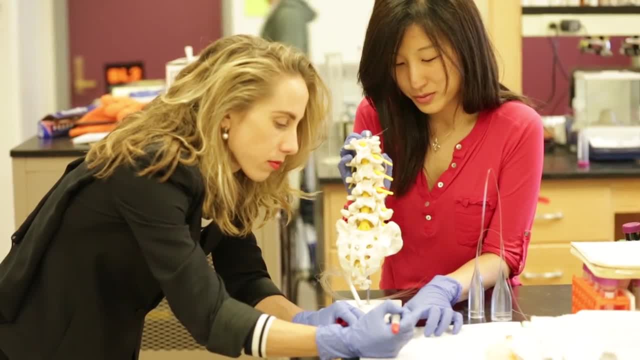 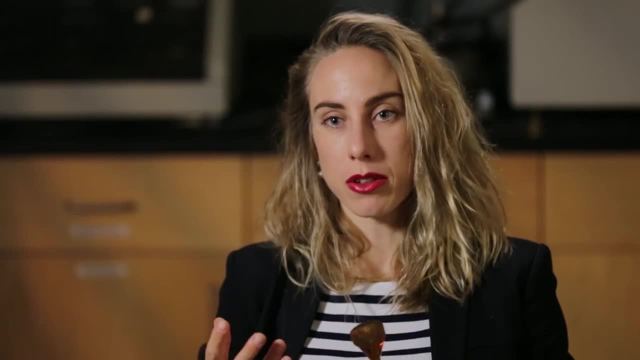 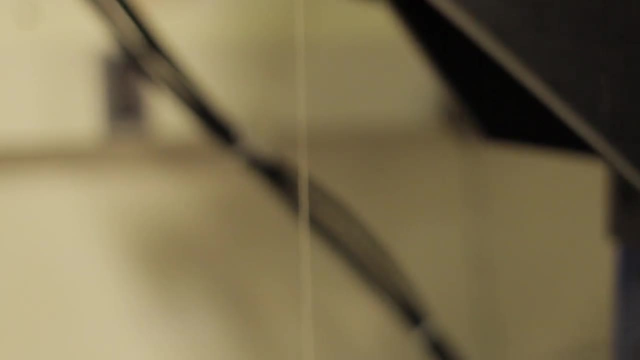 invasively. We are extremely excited what we were able to do with this technology, with this type of materials processing, because before we came into the field of neural engineering there was really no way of creating those complex multi-functional structures. And what 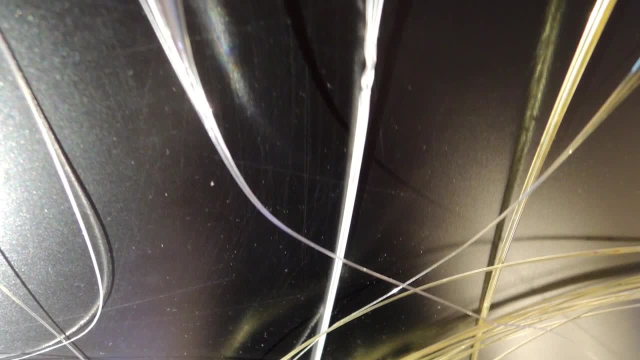 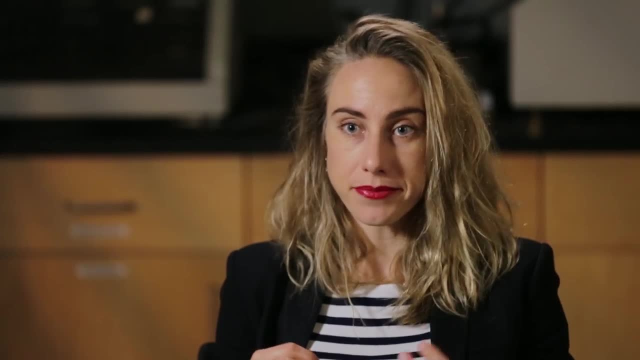 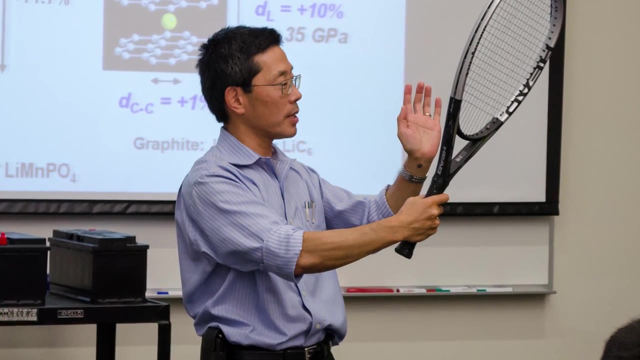 multi-material fiber technology allowed us to do is to incorporate all of those different modalities into a structure that is still very sleek and very biocompatible. Energy research in general offers tremendous opportunities for material scientists and engineers such as myself. Right now, one of the things that really fascinates me is whether 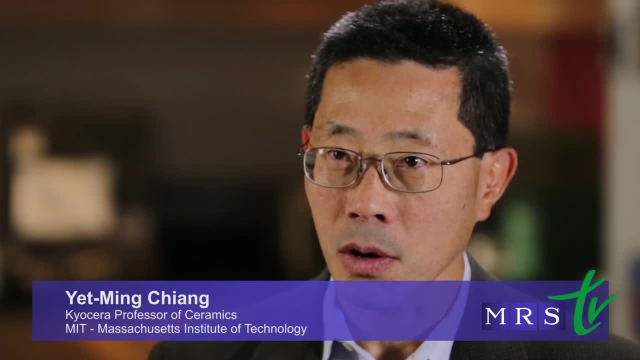 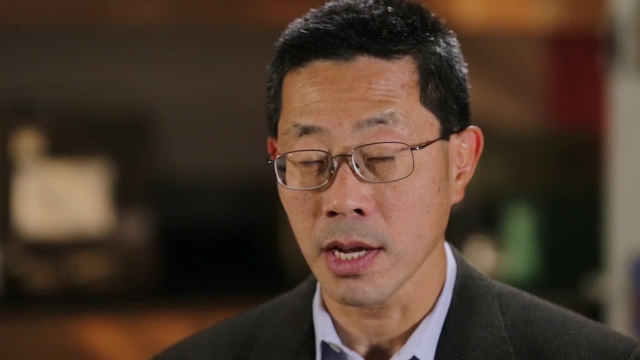 or not we can get the cost of energy storage down to a very low cost, So low that we can have a technology that enables not just the hourly shifting of something such as solar energy, not even daily, weekly, but actually seasonal shifting, So that for 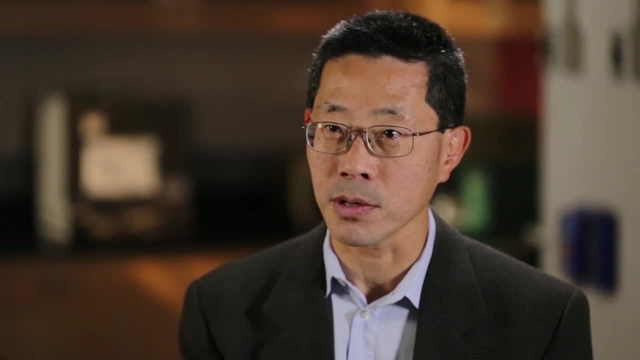 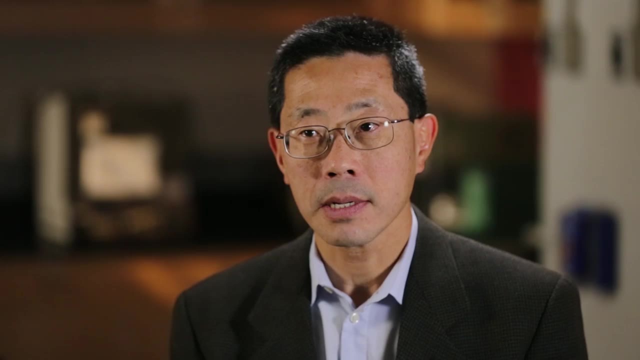 instance, in the Northern Hemisphere, where we have so much more sunlight in the summer than in the winter, it would be possible to store energy seasonally: store it in the summer and actually use it again in the winter. That will require new battery technology of extraordinarily. 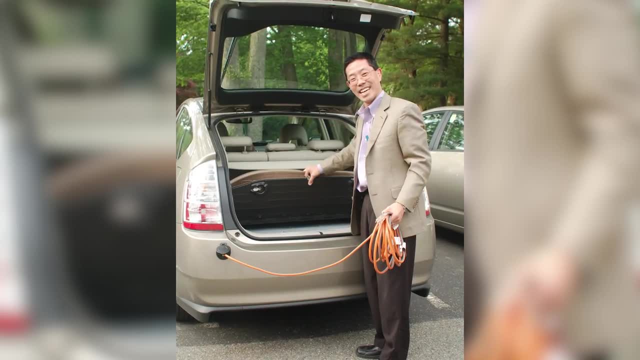 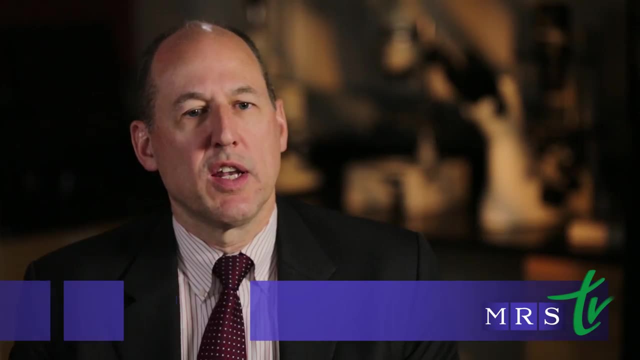 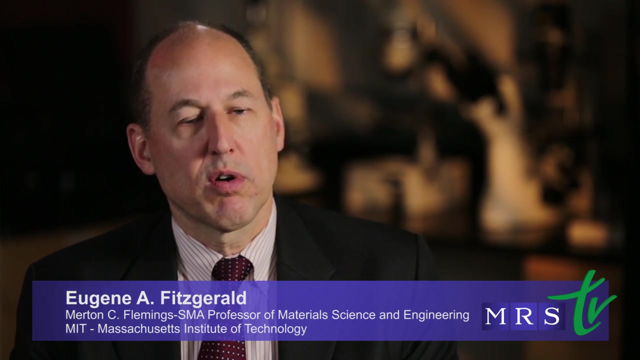 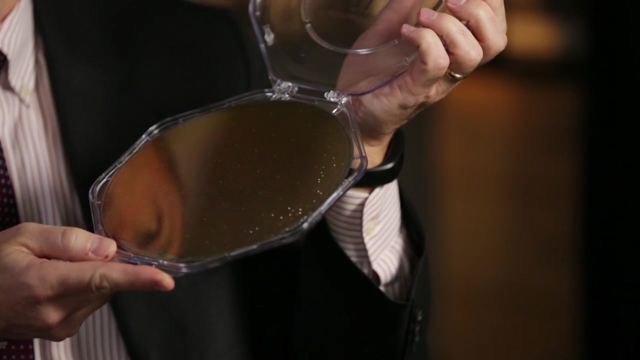 low cost and high performance. SMART is MIT's research lab in Singapore. It is designed to be a new experiment in international collaboration in areas of research that interest both Singapore researchers and MIT researchers. So an example of what we're doing, as shown here, is a 200-millimeter silicon CMOS wafer.